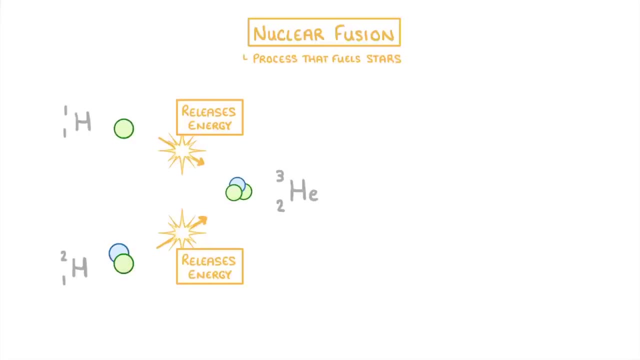 and is the process that fuels stars. It's also how all elements heavier than hydrogen were made. The reason fusion produces such large amounts of energy is that some of the mass of the original nuclei, in this case those two hydrogens, is being converted to. 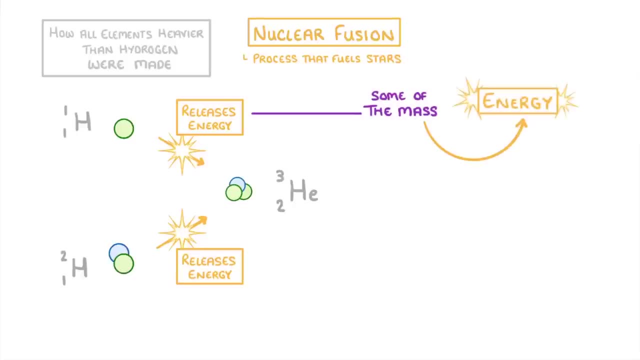 energy rather than transferred to the new helium nucleus. You can't tell this from looking at the mass numbers, but just trust us that the helium nuclei will be very slightly lighter than the hydrogen nuclei. You don't need to be able to calculate this energy in any way, but out of interest. 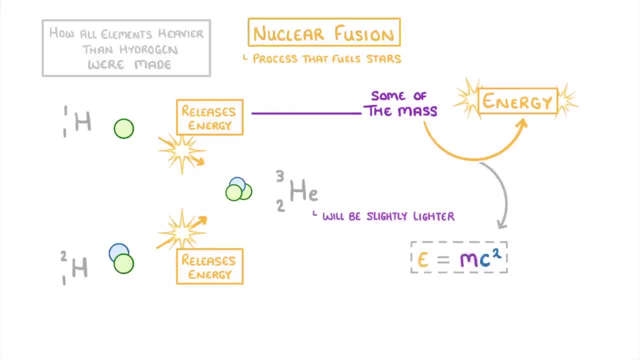 it is converted by Einstein's famous E equals mc squared equation, which tells us that you multiply the mass that's being lost by the speed of light squared to work out how much energy you'll be converted to. And as the speed of light squared is around 9 times 10, 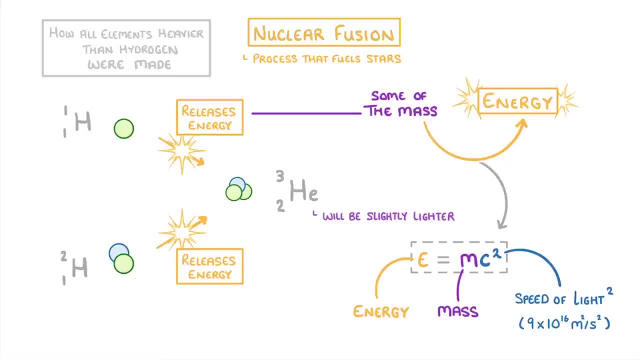 to the power of 16, you can see why a lot of energy is released. Another great thing about nuclear fusion is that it doesn't produce any radioactive waste, and we can easily make the hydrogen that's needed as a fuel. The issue, though: 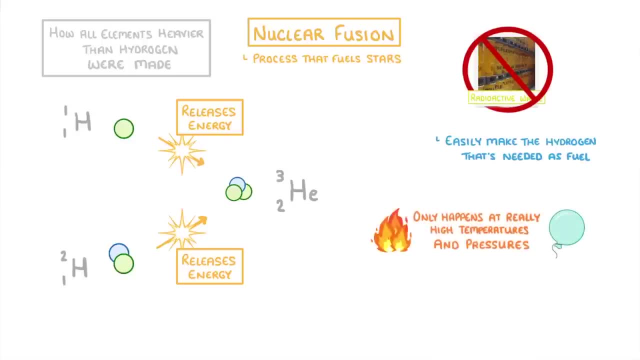 is that fusion only happens at really high temperatures and pressures, as in 10 million degrees celsius. Because of this we can't currently do nuclear fusion here on earth, but there is a lot of experimental research going into discovering how we could do nuclear. 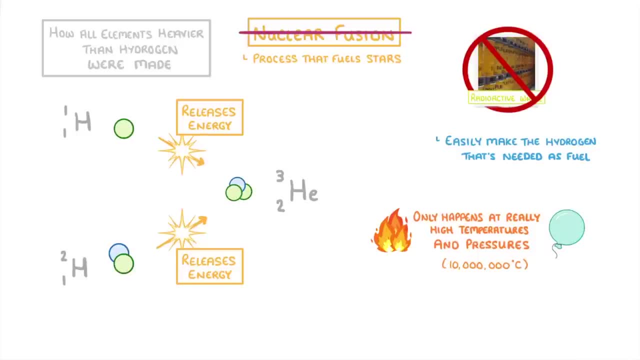 fusion here on earth. But there is a lot of experimental research going into discovering how we could do nuclear fusion here on earth and there is a lot of research going into discovering how we could do nuclear fusion here on earth, and there is a lot of experimental research going. 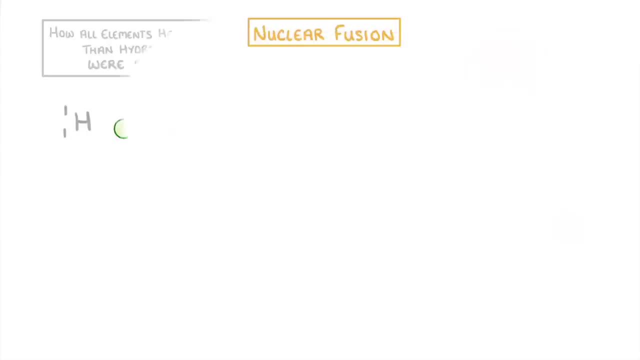 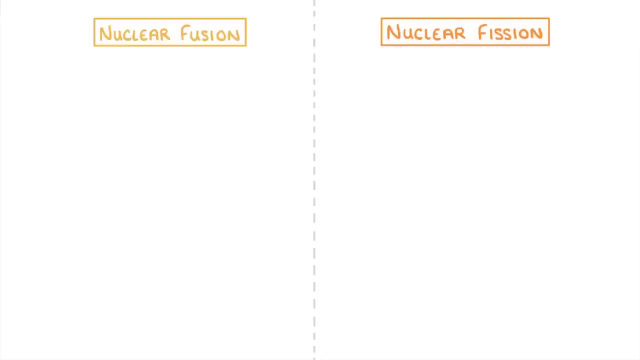 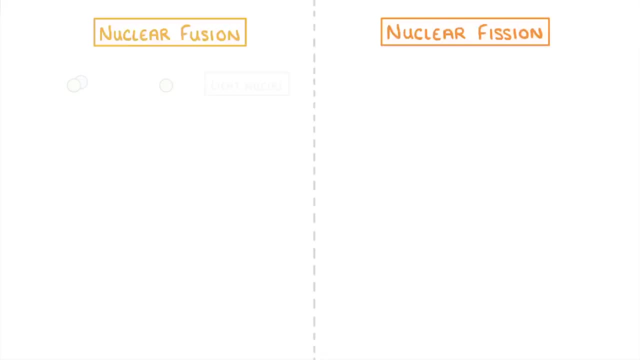 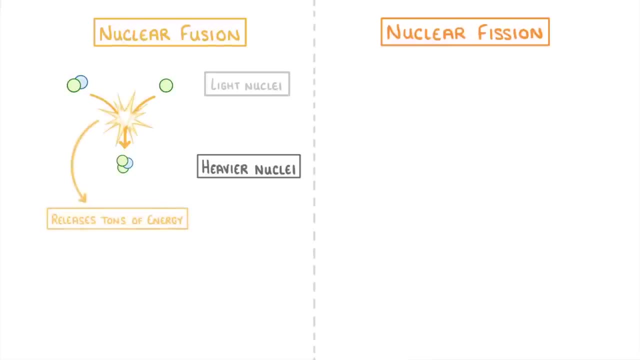